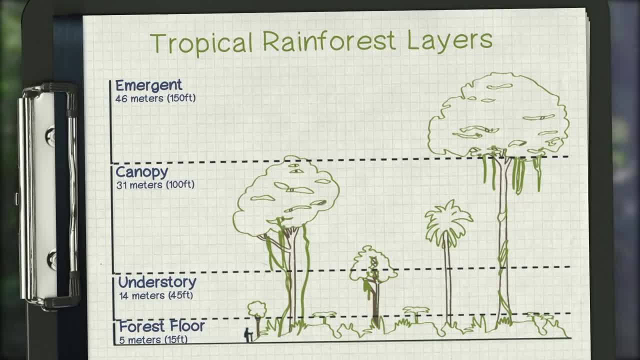 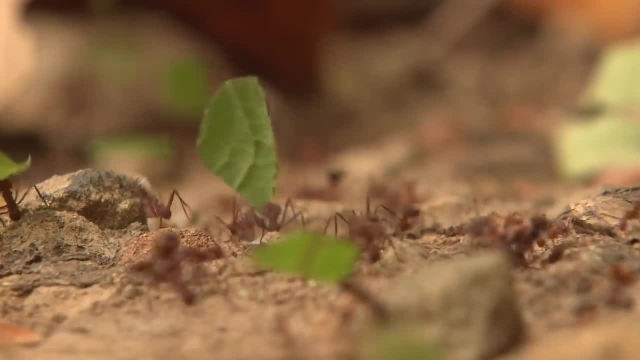 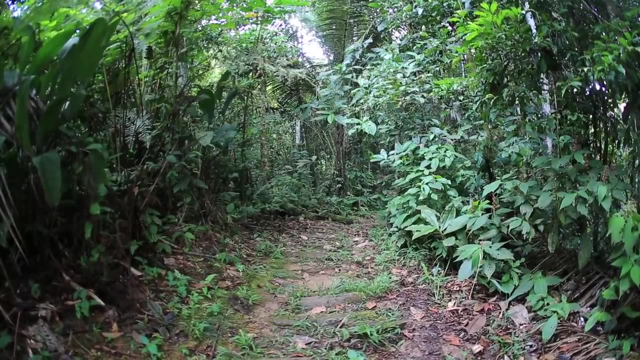 each with its own unique structure and composition. The forest floor receives very little sunlight. It is a hot, humid place where animals like leafcutter ants spend their time foraging for food. Just above the floor is a thick layer of shrubs, small trees and flowering plants. 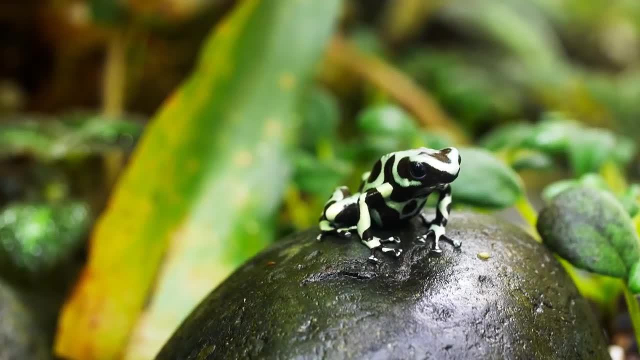 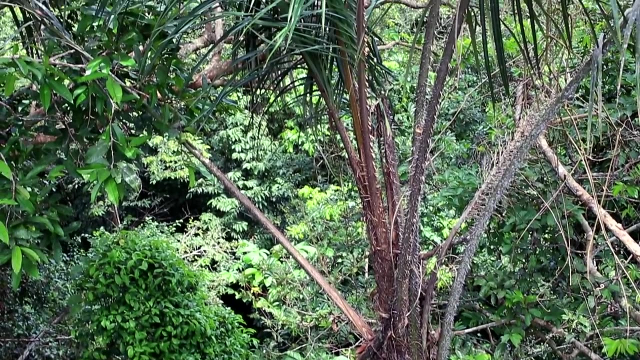 Here in the rainforest understory, you find amphibians like the poison dart frog, whose toxic skin protects it from predators. Rising higher, we find a bright connected layer of tree branches and leaves. The canopy contains a wide variety of species. 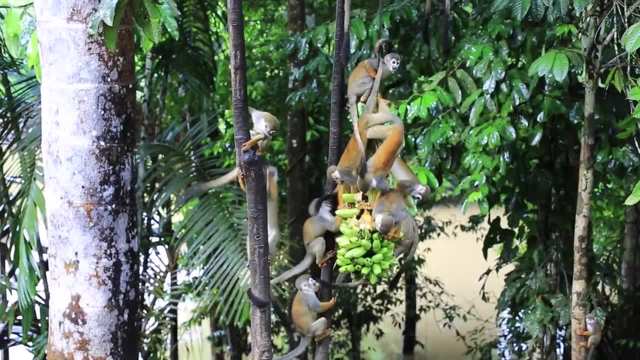 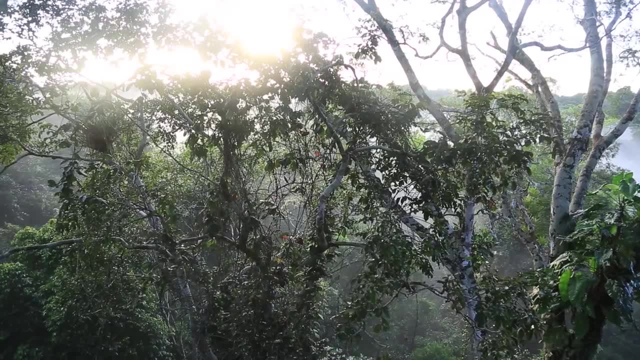 including squirrel monkeys, who travel and feed in large social groups. Breaking through, we enter the emergent layer, an open space containing only the highest treetop. Here we find camouflaged insects called katydids, who feed on young tender leaves. 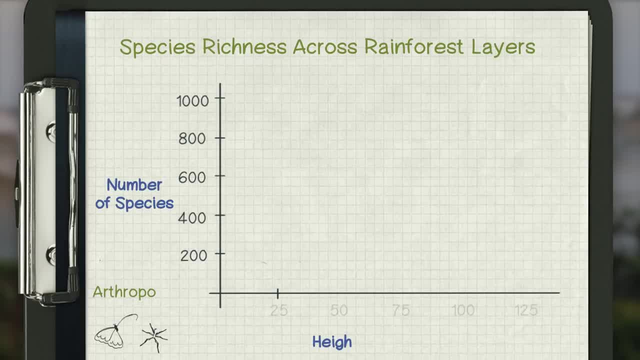 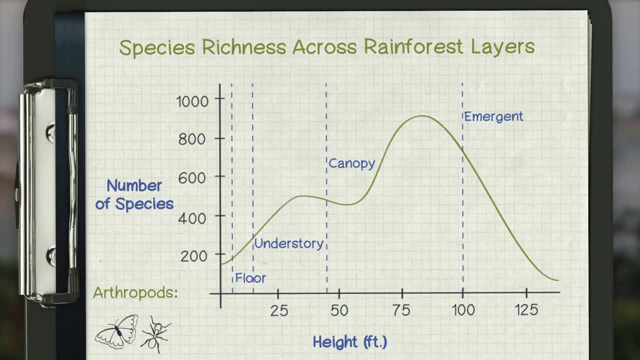 Now imagine you are a biologist researching arthropod diversity in the Peruvian rainforest. You and your team sample each forest layer, recording the number of species found and at white height, You and your team sample each forest layer recording the number of species found and at white height. 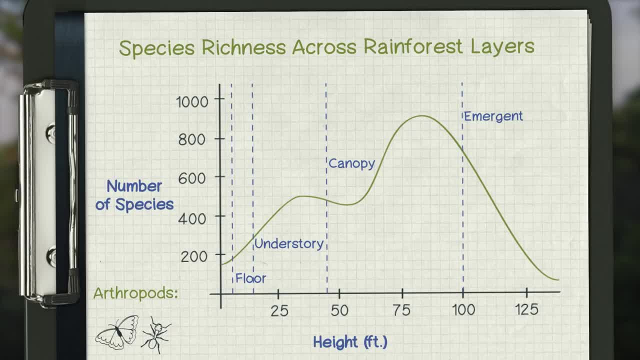 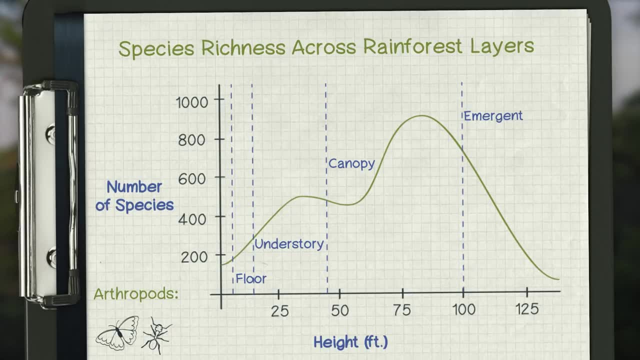 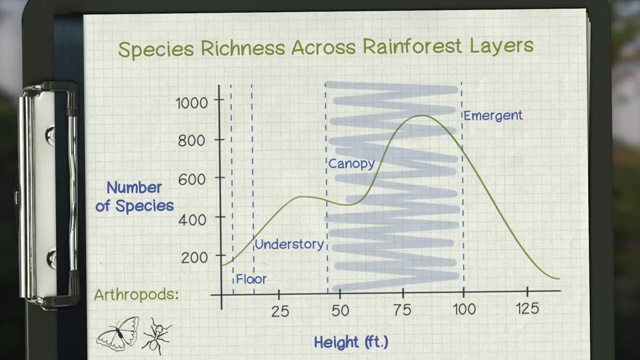 Looking over your field notes now. what trends do you see? How do the layers differ in species richness? Take a moment to pause the video and examine the graph. The canopy is believed to house over 70% of species found in the rainforest. 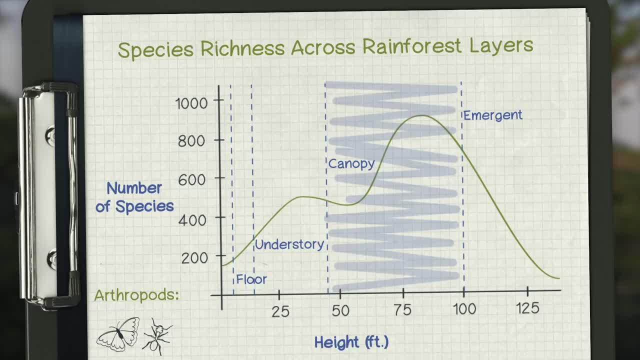 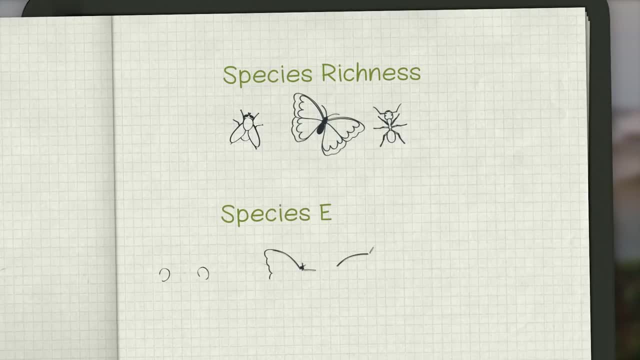 making it the most species-rich of the four layers. To measure species diversity, researchers like Michelle must take into account both species richness. to measure species diversity, researchers like Michelle must take into account both species richness, the number of different species and species evenness. 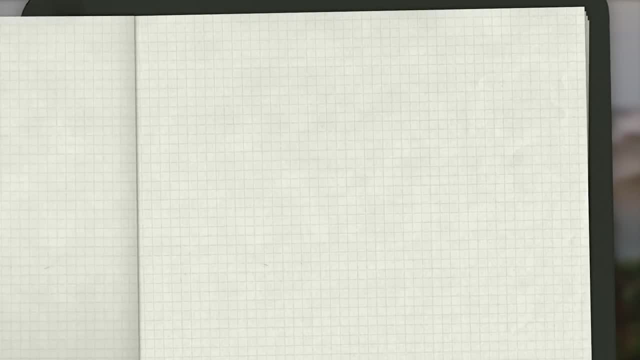 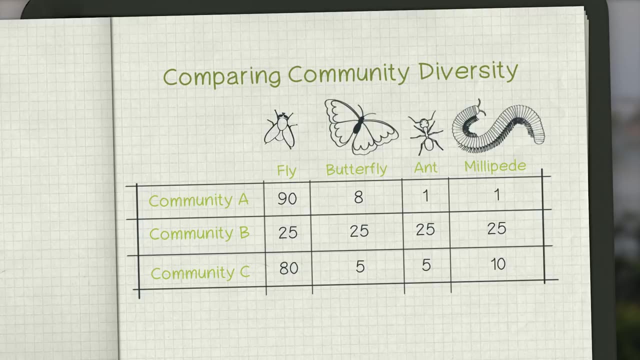 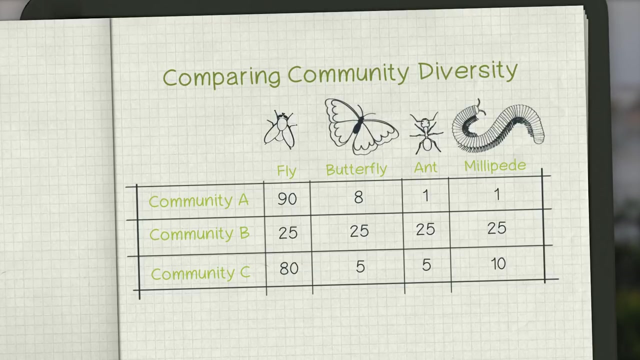 the abundance of each species. Imagine you survey three different rainforest communities and identify the following species at the following abundances: and identify the following species at the following abundances: Looking at your field notes now, which community appears to be most diverse? 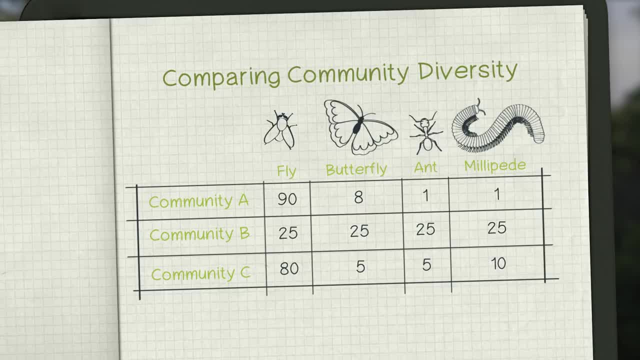 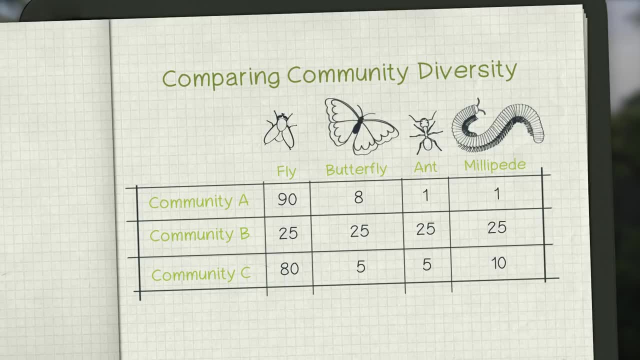 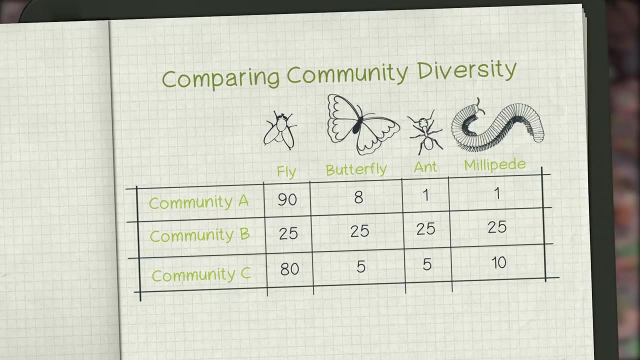 While each has the same number of species, Community B has greater evenness, a more balanced number of individuals from each species. We recognize Community B as being more diverse because of its high species richness and its high species evenness. Why is this important?